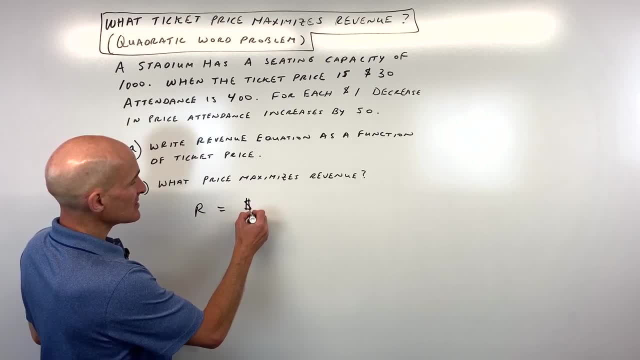 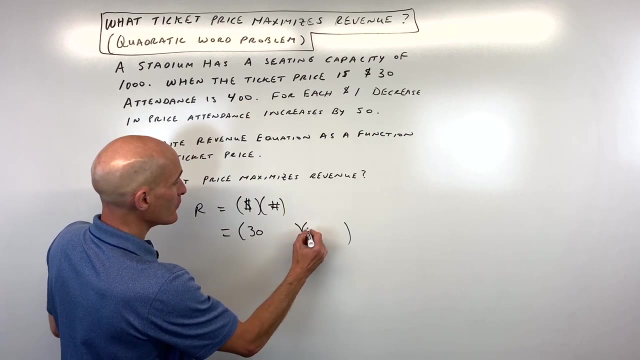 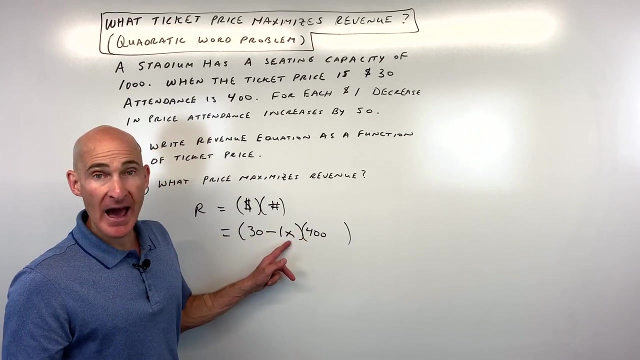 is what it's: the number of tickets, right, number of tickets times how much each ticket is. So let's see. so, in this case, how much is a ticket? right now, a ticket is thirty dollars, okay, and how many people are attending? four hundred people. But if you decrease the price by a dollar- and I'm going to write minus one, X- 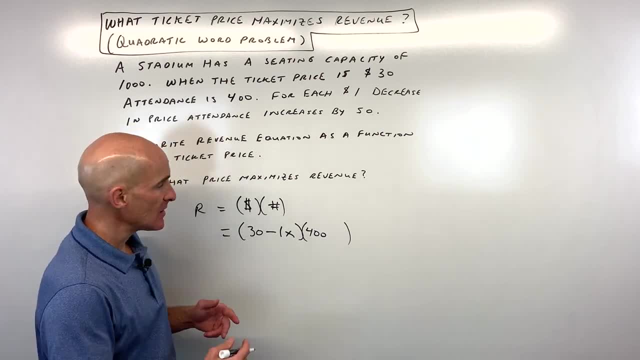 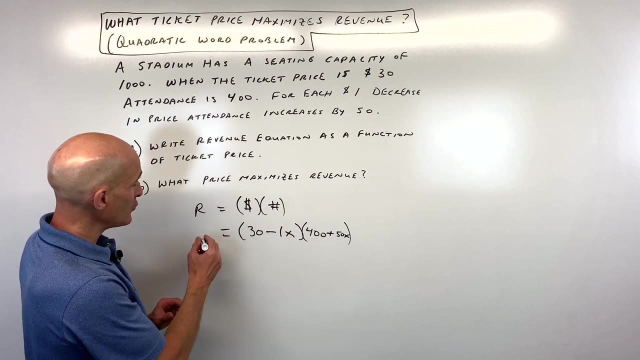 where x is the number of one dollar. price decreases, the attendance is going to go up by 50 times x. See, if you decrease two dollars, then two times 50 is 100. it goes up by 100 people now people attending. Okay, so now we have our revenue equation as a function of X, the number of 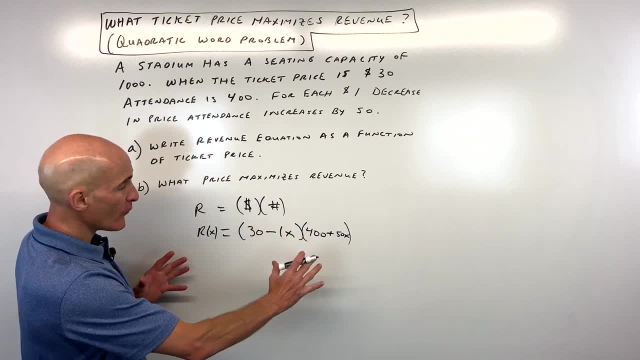 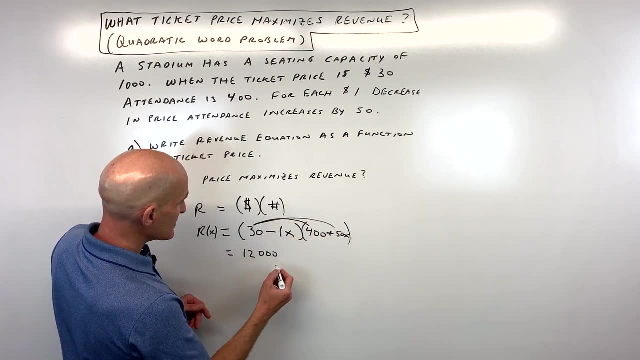 decreases in the price by $1.. But let's go ahead and FOIL this out. So we have 30 times 400,, which is going to be 12,000.. We have 30 times 50, which is 1,500 X. We have negative 400 X. 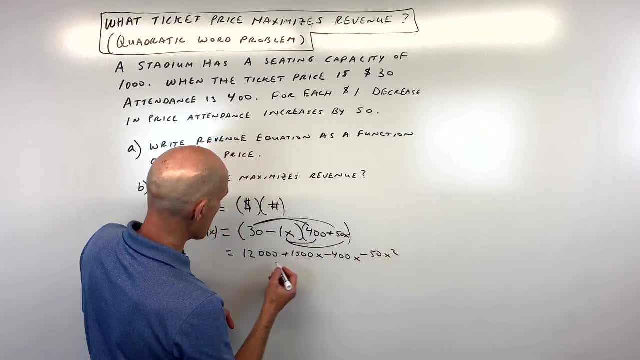 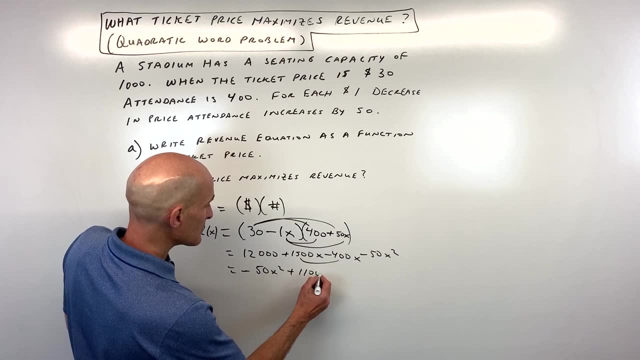 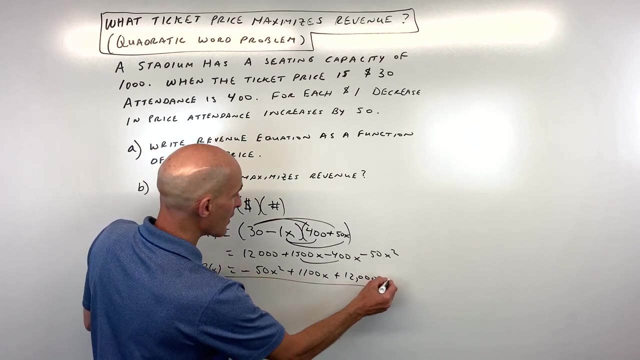 and we have negative 50 X squared. Let's put this in descending order. So we have negative 50 X squared. This comes out to 1,100 X and plus 12,000.. Okay, so that's our revenue equation. right there, That's part A. Now part B. what price maximizes the revenue? Well, one thing I. 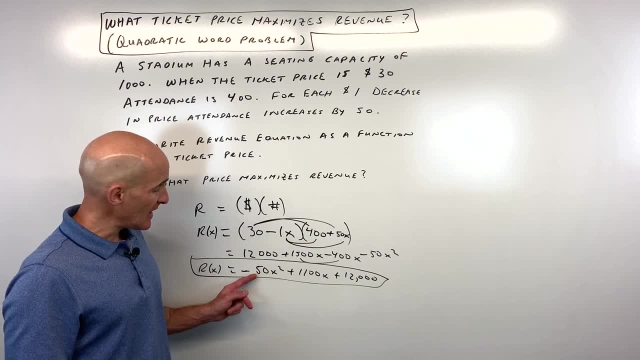 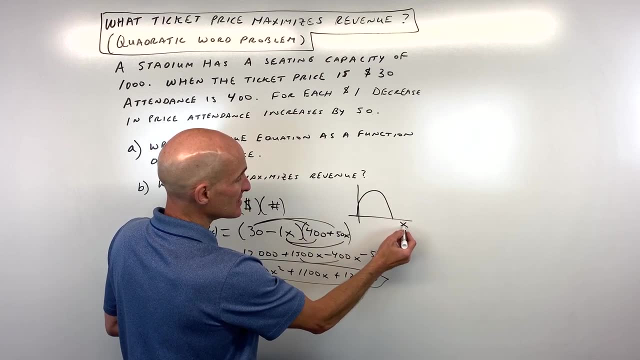 want to point out. this is a quadratic. see X squared, But notice the A value is negative. So what does that tell us? The parabola is opening down right. So here's the number of price decreases, Here's your revenue, And we're trying to figure out. 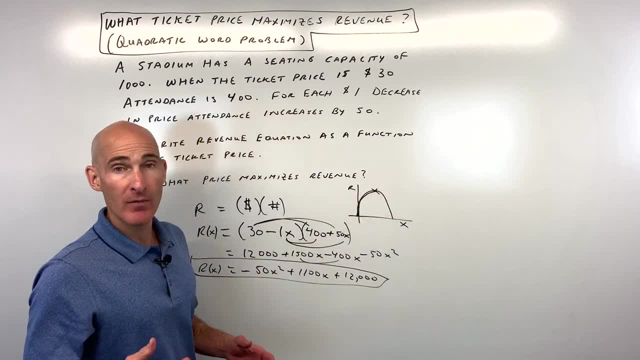 the value of the revenue. So we're trying to figure out the value of the revenue. So we're trying to figure out the value of the revenue. So we're trying to figure out the value of the This point, right here, where it's a maximum point, And because that A value is negative. 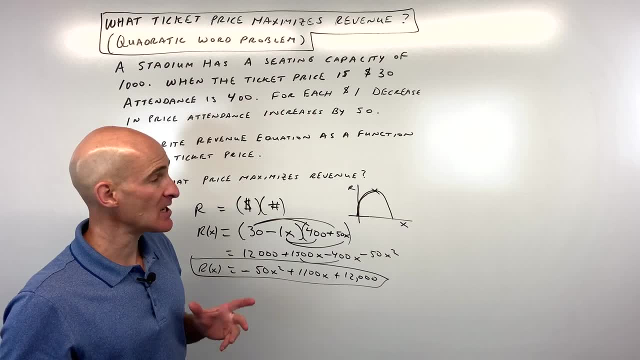 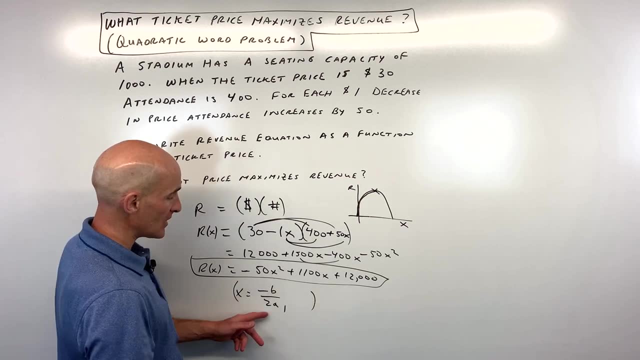 it opens down right So that maximum is going to be at that vertex. And you know the formula for finding the vertex: X equals negative B over 2A. That'll give us our X coordinate And that would represent the number of $1 price decreases. If we solve for the Y coordinate, that's going.